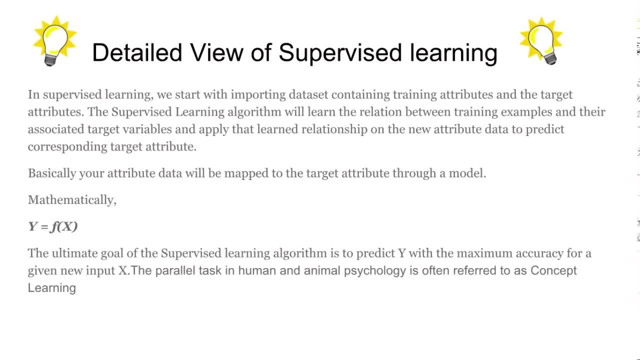 example for it and then provide you question to solve. In similar fashion, for computers, we use to provide training attributes along with target attributes. This phase is known as training, And in supervised learning, we use to provide data set in which we give training attribute. 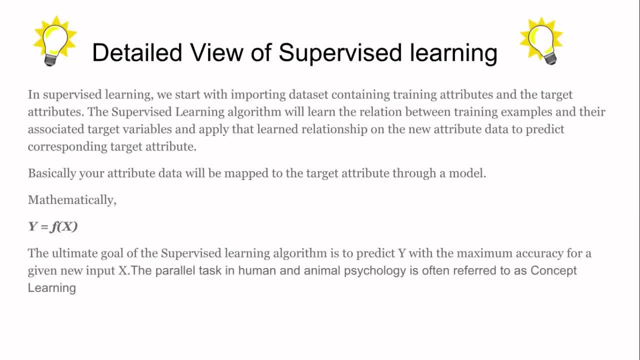 and as well as target attribute, such that each training example is associated with their target label, And we apply that learning relationship on the new attribute data to predict the corresponding target attributes Mathematically, we use to formulate a function f such that it maps: 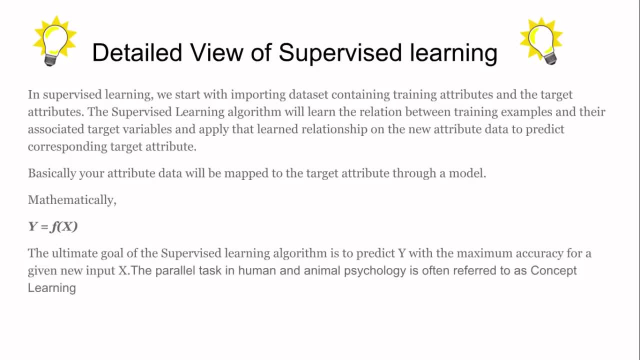 from training attributes to target attributes, that is, from x to y, And then, after we get that function, we use to take some unknown examples, that is, unknown x, and use to predict y. for the same, The ultimate goal of the supervised learning is to predict y with the maximum accuracy. 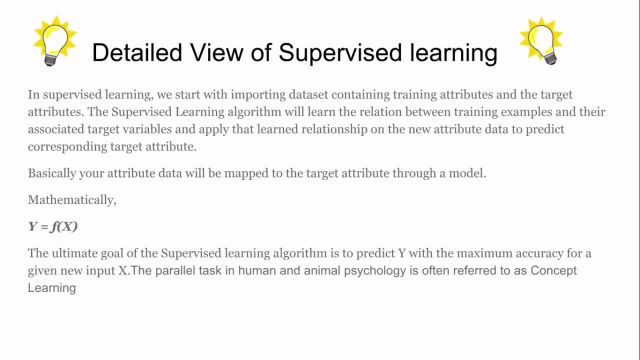 given the new input x And how we will calculate it. We first calculate function f such that it properly maps x with y for the training example. And after getting that function which properly maps with x to y, Then we use to test it on the testing phase and use to predict the actual y for any unknown. 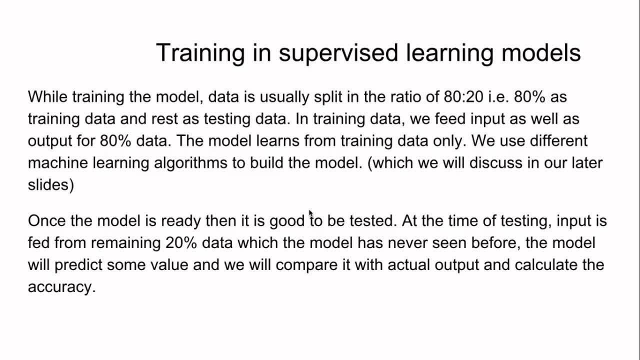 training attribute. So for training we have 80 to 20% ratio in which 80% is training data and rest is testing data. So we use to feed 80% of input data as a training phase and 20% as a testing phase, and basically 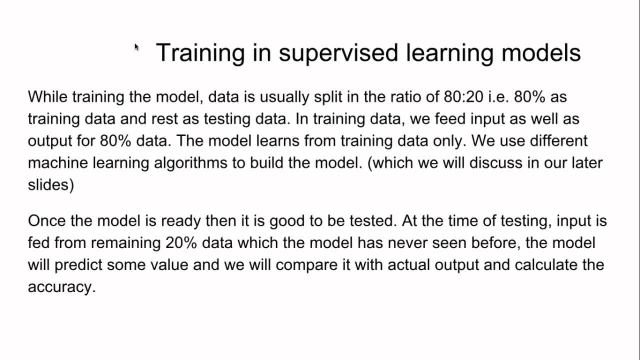 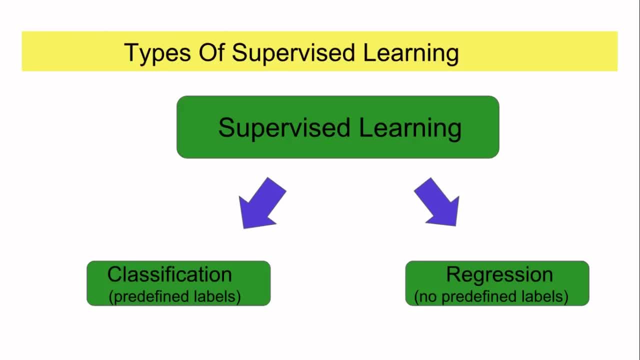 check And then we use to test it on the testing phase and use to predict the actual y for the training example. So this is how the supervised learning works. So the supervised learning is basically a model using this remaining 20% data. So basically, supervised learning are of two types: classification and regression. 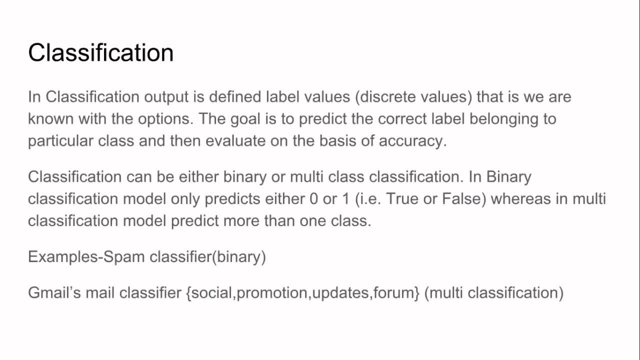 In classification we basically classify what type of output it is, whether it belongs to some class 1 or class 2 or class 3.. For example, we can have an example of binary classification, example: spam classifier. So in spam classifier we use to classify the data. 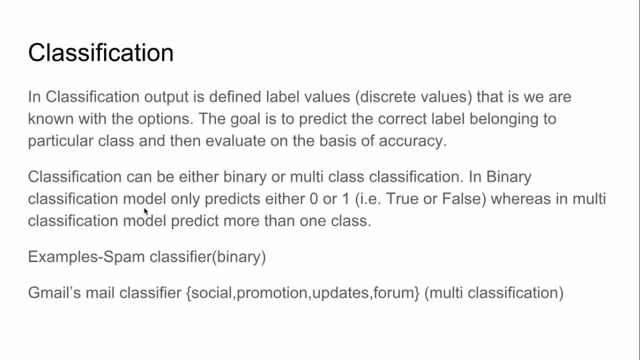 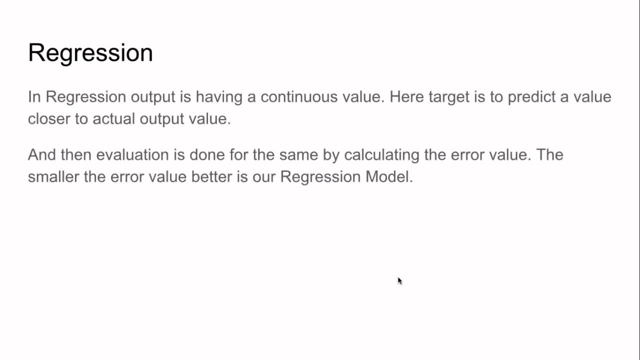 For example, we can have an example of binary classification, example: spam classifier. For example, we can classify that the email is spam or not. Nowadays, Gmail has a multi classification for classifying mail, such as social promotion, updates and form, So it classifies more than one category. hence it is a type of multi classifier.